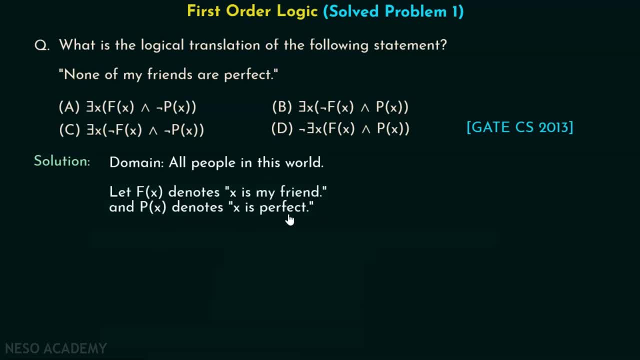 f denotes x is my friend and p denotes x is perfect. Okay, so here f denotes x is my friend and p denotes x is perfect. So none of my friends are perfect. can be translated to for all x. f implies not of p. 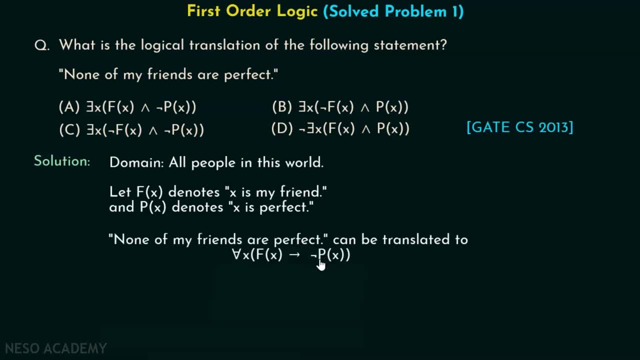 Isn't that? so We can easily write this statement, because here we are talking about: none of my friends are perfect. That means my all friends are not perfect, Right? so here this is for all. x, Of course, for all. quantifier will come into picture. 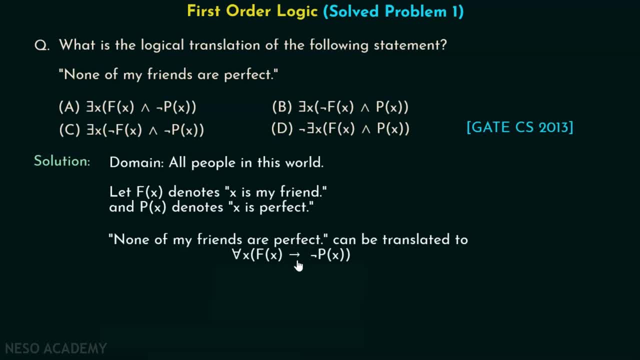 We are talking about all the people in this world. that is why implication is required, because here I have to select my friends Right. So if x is my friend, then x is not perfect. That is what this statement means. So, for all people in this world. 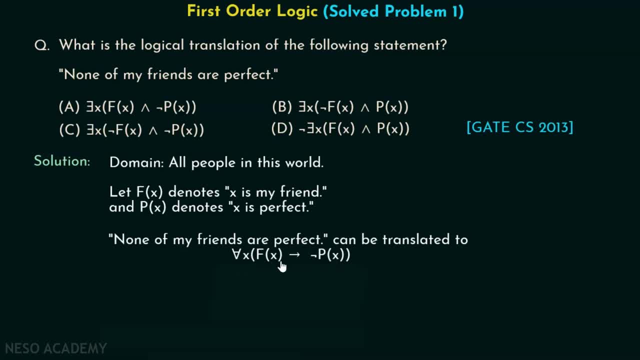 if x is my friend, then x is not perfect. Now here we can write this as not of f or not of p, because here we can easily convert this p implies q form to not of p or q. So here we can write: 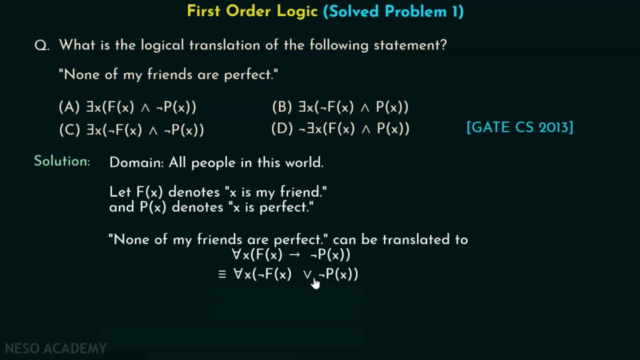 not of f or not of p, And then after that we will move this negation outside So this becomes not of f and p, And finally, we can move this negation one step towards left so that this becomes not of their exist: x, f and p. 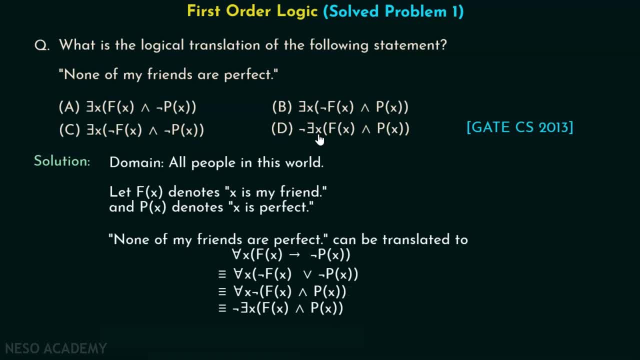 You can see over here that option D is straight away the correct option. that is not of their exist x, f and p. It says that it is not the case that there is some of my friend who is perfect. This is the same thing, right. 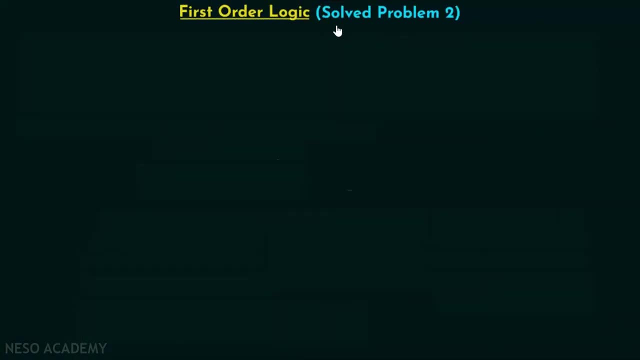 So option D is the correct option. Let's discuss, solve problem two, on first order logic, Which one of the following is not logically equivalent to: not of their exist: x, for all y alpha and for all z beta. We have to find out which one of the following: 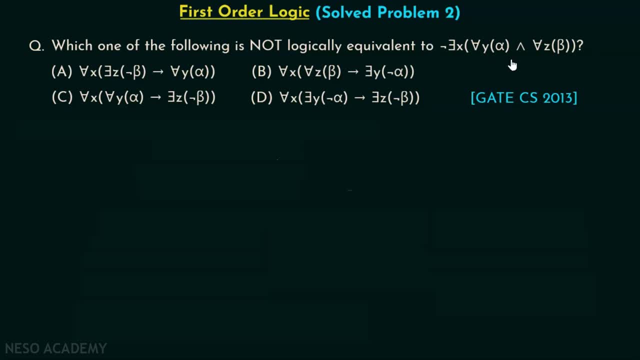 is not logically equivalent to this particular logical expression. Okay, So these are the options available in front of you, And this question has been asked in GATE CS 2013.. I would encourage you to pause the video for a while and try to answer this question on your own. 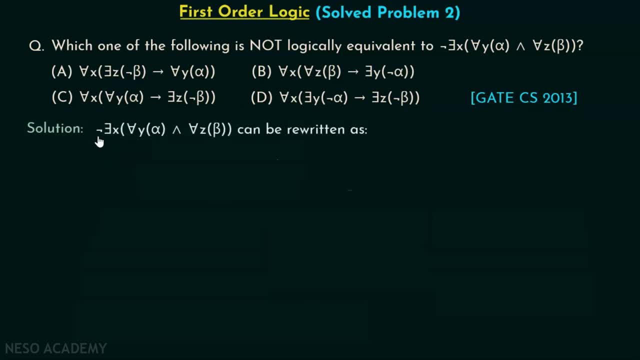 I hope you are done. Okay, let's move on to the solution. This particular logical expression, that is not of their exist x for all y alpha and for all z beta can be rewritten as for all x, not of for all y alpha and for all z beta. 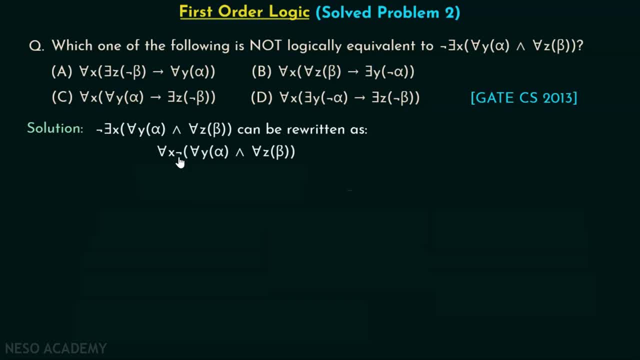 I have just moved this not towards right. That's what I have done, And then again, I will move this not towards right. So this becomes not for all y alpha, This becomes or, and this becomes not for all z beta. After this, I will move this not towards right. 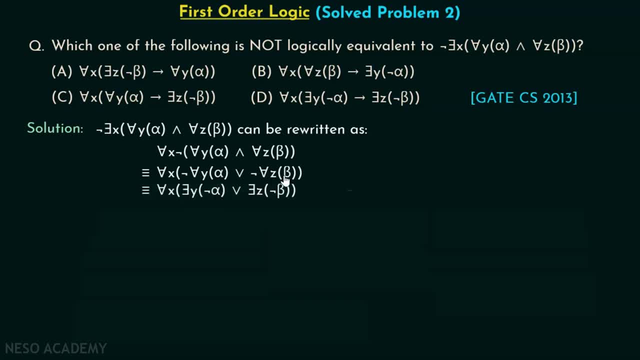 This becomes: there exist y not of alpha, and also this not towards right. So this becomes: there exist z not of beta. So this is the final expression so obtained. Now let us consider these options one by one. Option A For all x: there exist z not of beta. 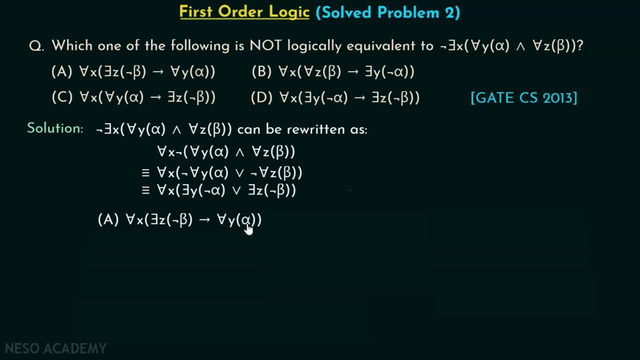 implies for all y alpha. We need to write this particular expression in this form, And this can be written by converting this implication to its equivalent form, that is, p implies q can be converted to not of p or q. Right, I will just write: not of. there exist z, not of beta. 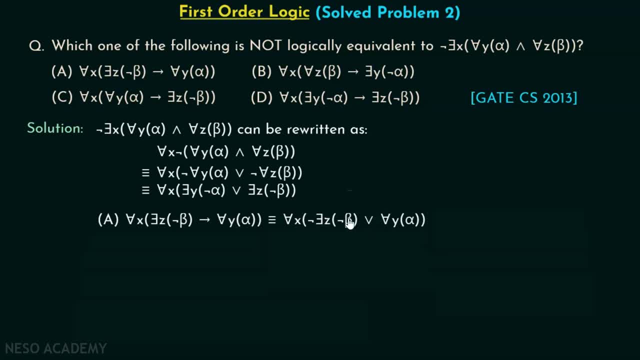 or for all y alpha. If I move this not towards right, then this becomes for all z beta or for all y alpha. This is definitely not equivalent to this particular expression. So obviously option A is the correct option. Let's see option B as well. 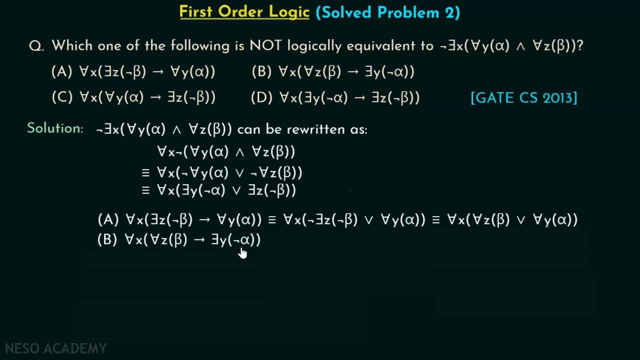 This is for all x, for all z beta implies there exist y, not of alpha. Obviously I can write this in this form: not of for all z beta, or there exist y, not alpha. Here I will just write and move this not towards right. 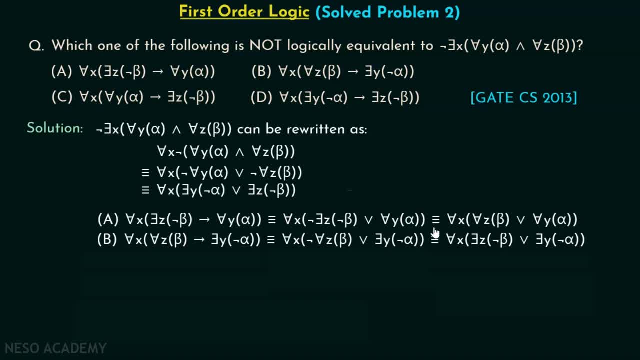 So this becomes: there exist z, not of beta. Now you can see this logical expression is equivalent to this expression. Obviously, this order is changed, but they are equivalent. Right, Let's see option C For all, x for all y, alpha. 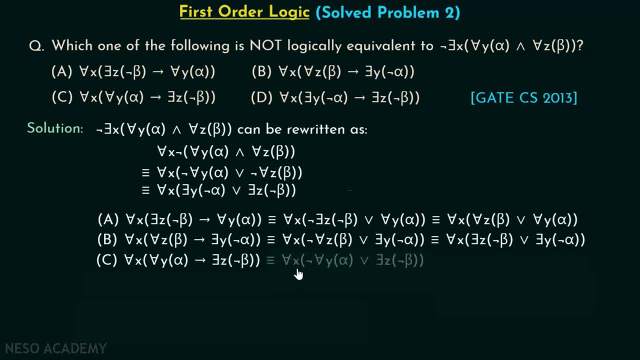 implies there exist z not of beta. This can be rewritten as for all x, not for all y alpha, or there exist z not beta. We can move this towards right. So this becomes: there exist y not of alpha, or there exist z not beta. 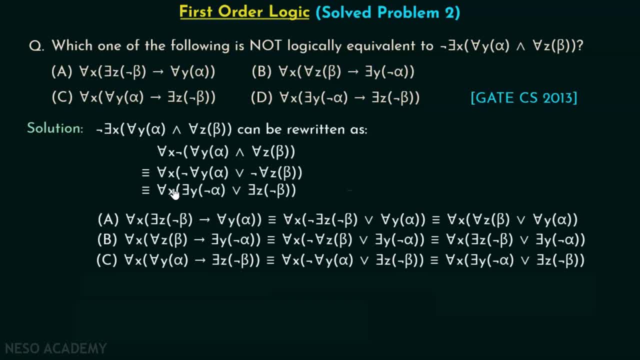 Obviously this is equivalent to this particular expression. Now let's consider option D. That is, for all x, there exist, y, not alpha, implies there exist z, not beta. Now, here again we can rewrite this: as for all x not of there exist y not alpha.